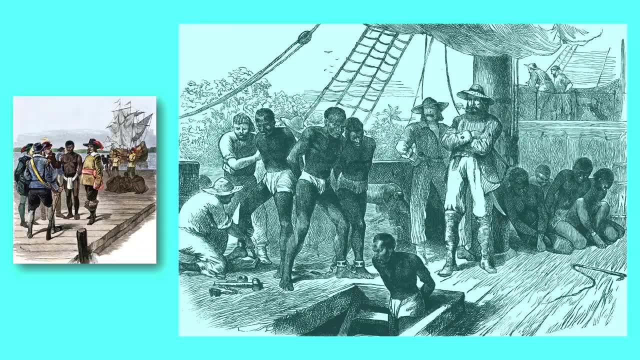 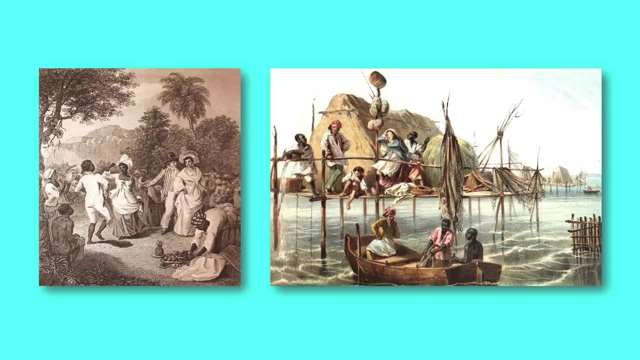 more Africans would be forced to migrate to Virginia to become slaves. What's weird is that in those early years, some slaves could wander freely, get married, buy land and other property or even buy their own freedom. Yep, that means they were actually getting paid some for their 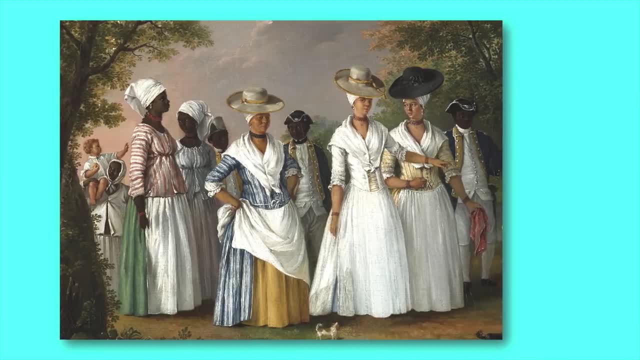 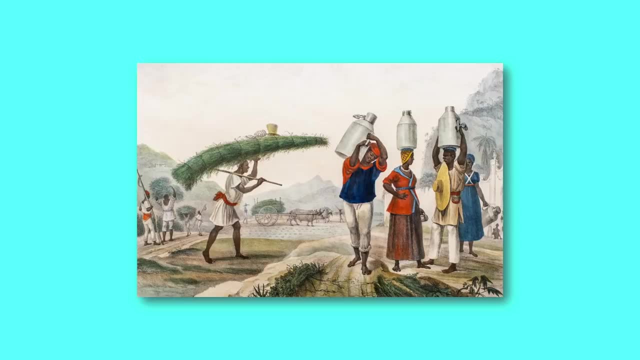 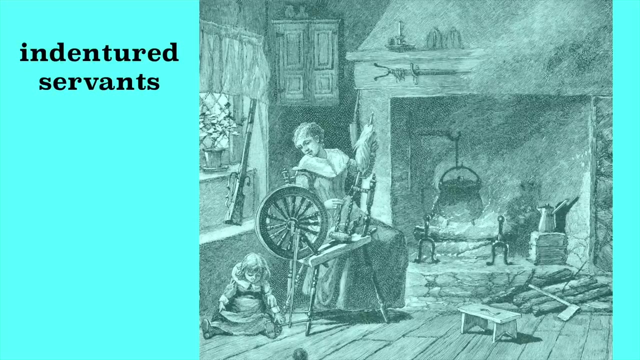 work And several Africans in Virginia were not slaves. In one Virginian county in 1660, in 1668,, 29% of all Africans were free. At least one African American had an indentured servant at one point. Oh yeah, indentured servants, or people who paid for their passage. 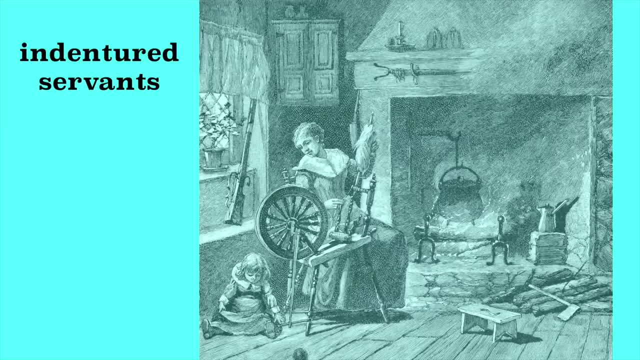 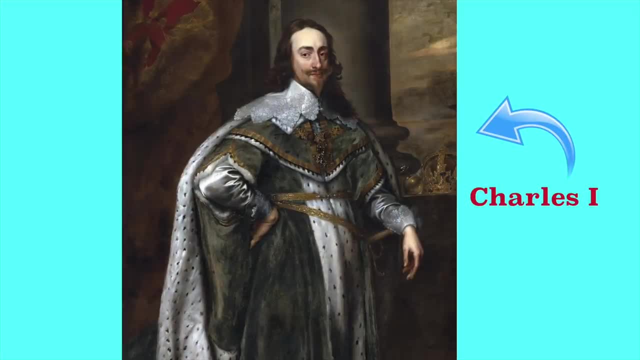 to the Americas by being forced to work for somebody for a certain number of years before getting their freedom, were also very common in the colony of Virginia, especially after King Charles I's supporters came to Virginia in large numbers after he died in 1649.. Beginning: 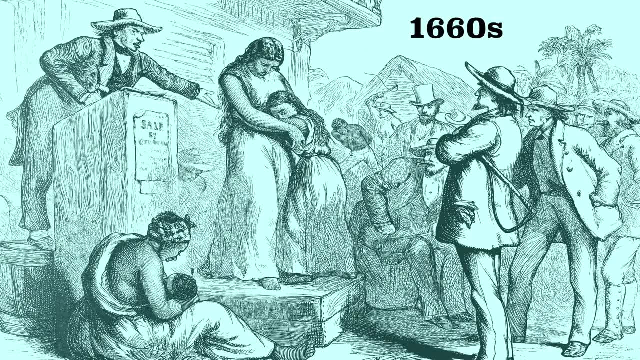 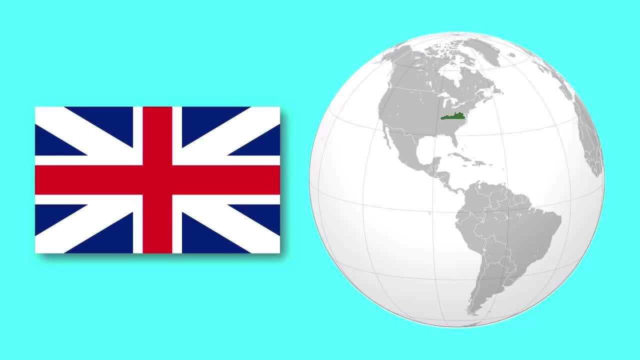 in the late 1660s, Virginia colonists would sadly pass new laws that further restricted the rights of all blacks, both free and slaves. Meanwhile, the British Crown had taken over the colony of Virginia, since they didn't like how the London Company was running things. 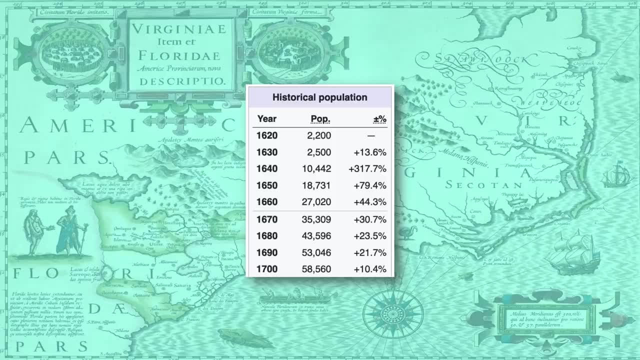 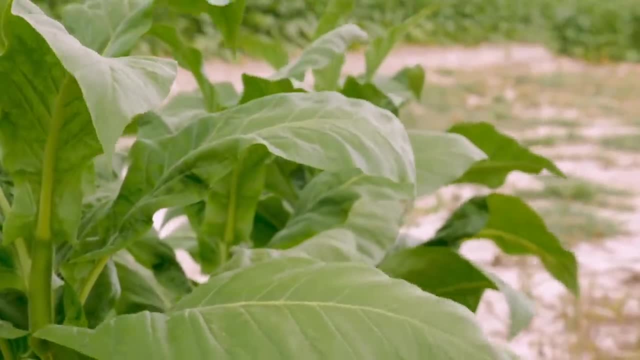 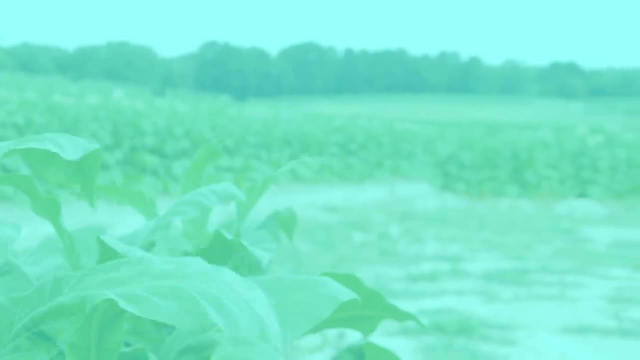 For the rest of the 1600s the colony grew quickly and brought a lot of wealth to England and certain plantation owners. Most of this wealth was concentrated in the hands of a few elite folks in East Virginia, But in Western Virginia farmers were barely getting by. One farmer out there, a dude. 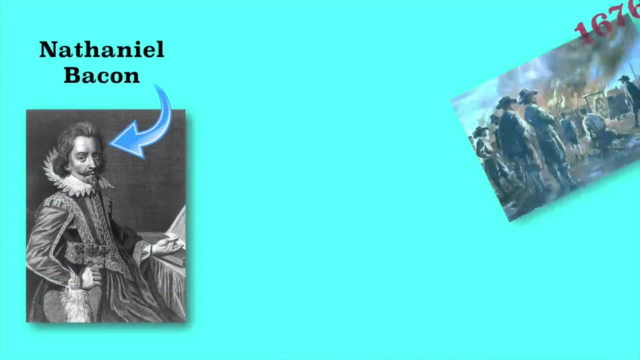 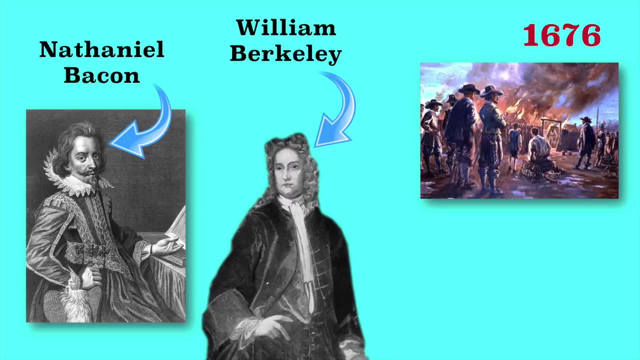 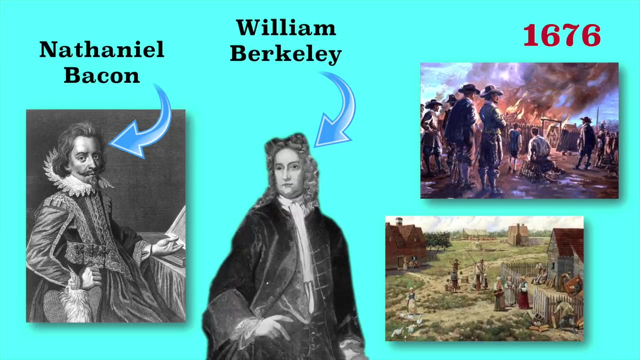 named Nathaniel Bacon, helped launch a rebellion in 1676 against Colonial Governor William Berkeley, mostly due to this huge economic inequality, but also since Berkeley wasn't doing much to protect farmers, constantly being attacked by American Indians. Now, why were American Indians attacking these farmers? Well, you know, since the farmers were taking 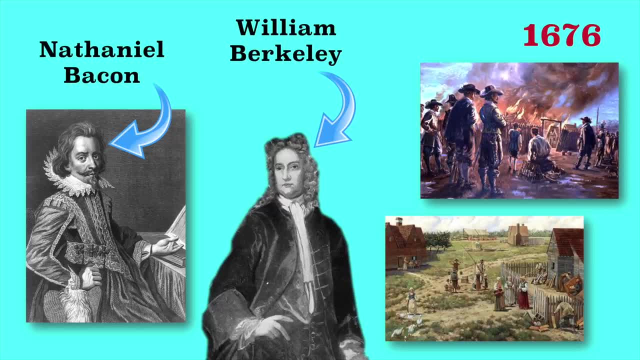 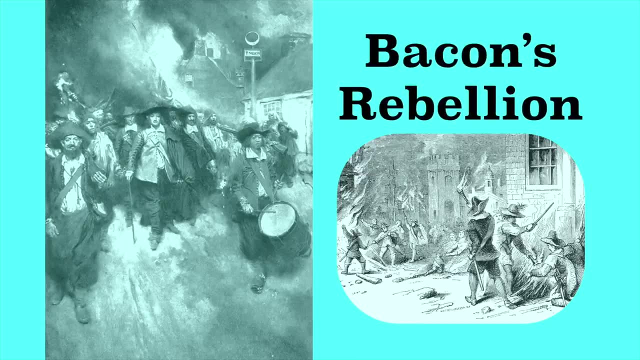 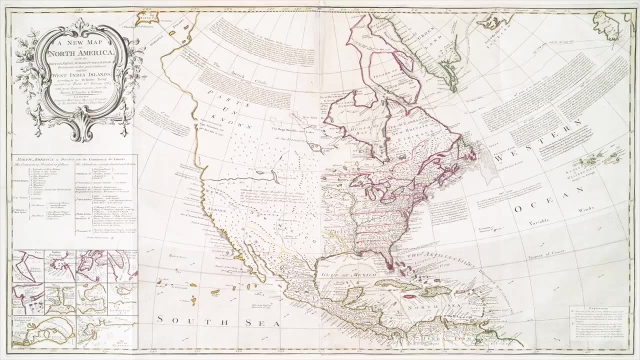 their land And had been for decades. But regardless, Berkeley seemed to be on the American Indian side, and so rebellion. even though what became known as Bacon's Rebellion failed, the tension between Eastern and Western Virginia did not go away. Let's flash forward to 1763. As a result of the Treaty of Paris that ended the French 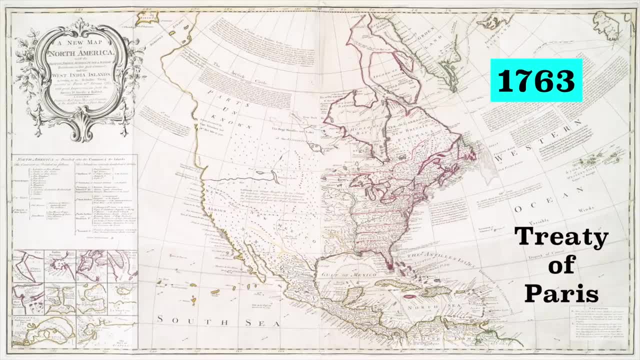 and Indian War. Britain took control of territory beyond Western Virginia in the Ohio Valley With the Proclamation of 1763,. the French and Indian War ended and Britain took control of territory beyond Western Virginia in the Ohio Valley With the Proclamation of 1763,. 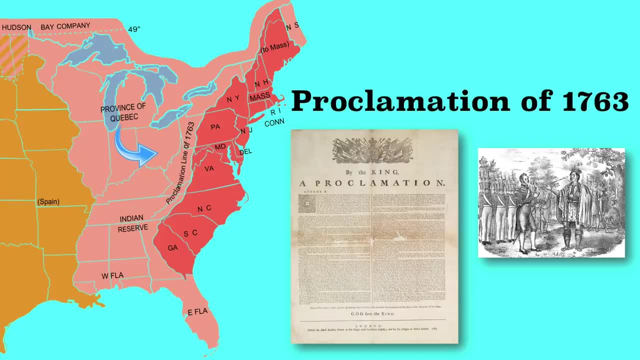 Britain took control of territory beyond Western Virginia in the Ohio Valley With the Proclamation of 1763,. the French and Indian War ended With the Proclamation of 1763,. it also established a boundary banning colonial settlers from moving west of it to appease American Indian. 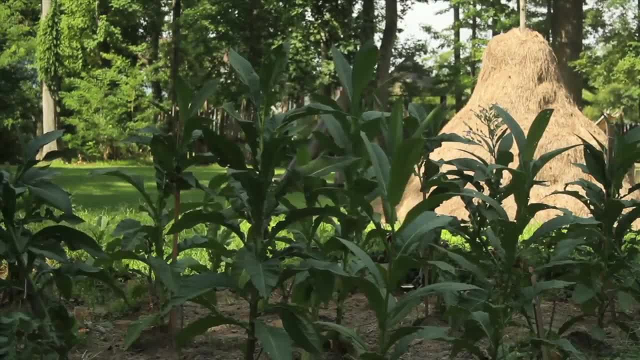 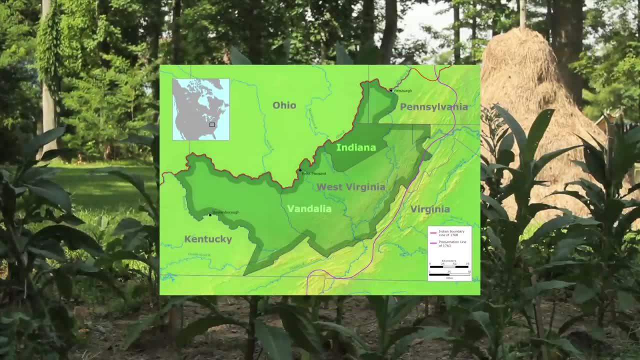 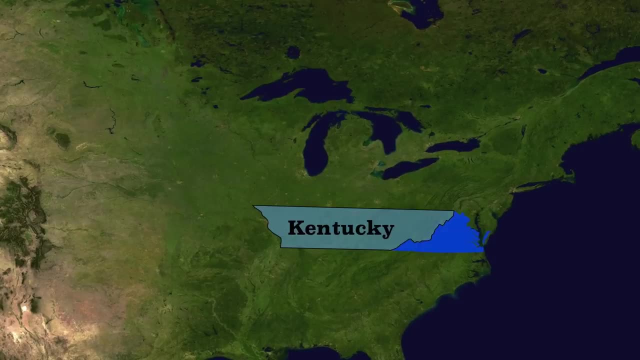 tribes. However, some Western Virginia pioneers were like nuh-un and settled west of the proclamation boundary anyway. Some even called for a new colony out there called Vandalia. Virginia had to respond and established a county out there called Kentucky during the 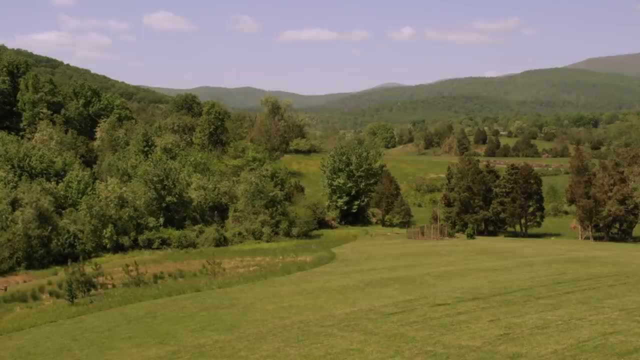 American War of Independence, But it had a hard time keeping track of what was going on out west. But it had a hard time keeping track of what was going on out west. This was a new colony, especially since once you got into the mountains it was harder to get around. 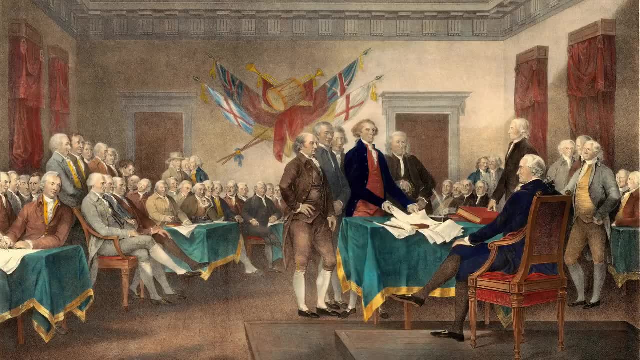 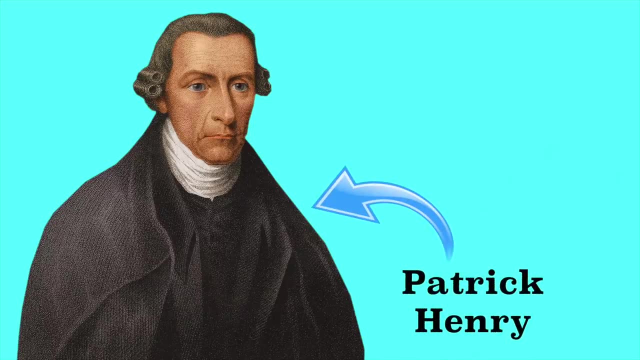 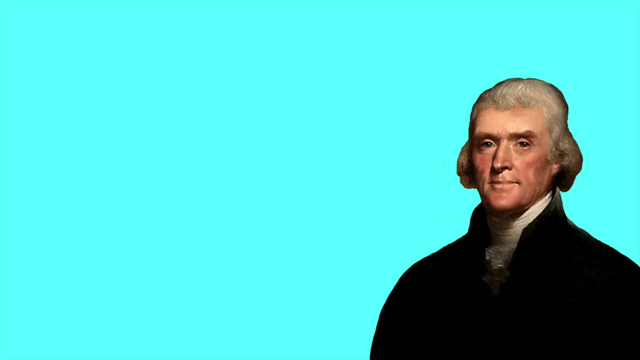 Back to the American Revolution. Um yeah, Virginia and its citizens played a big, freaking part, Like this dude, Patrick Henry, a future governor of the state of Virginia, but more famously known as the quote give me liberty or give me death speech guy. And this dude. 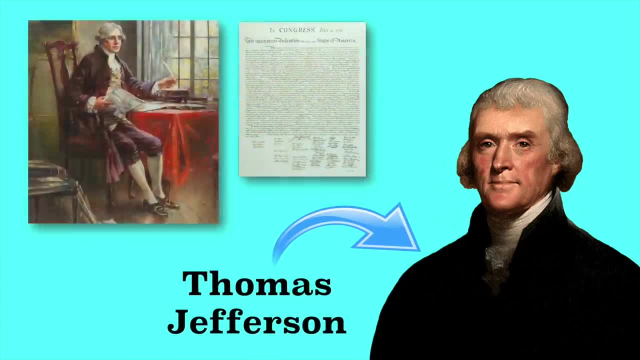 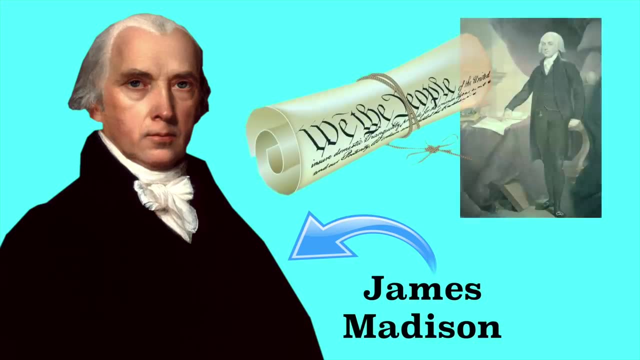 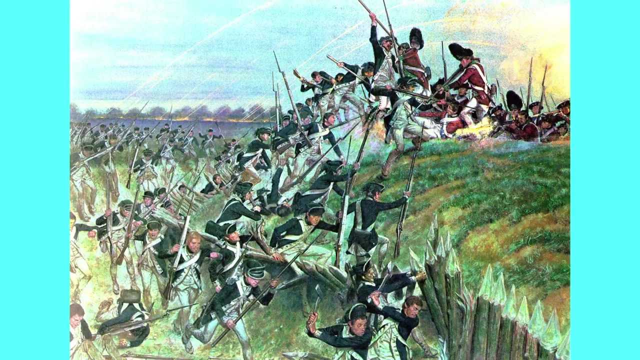 Thomas Jefferson, who I don't know was the main writer of the Declaration of Independence. Or this dude, James Madison, who I don't know was the main writer of the United States Constitution. Many of the soldiers who fought and many of the generals who led in the war. 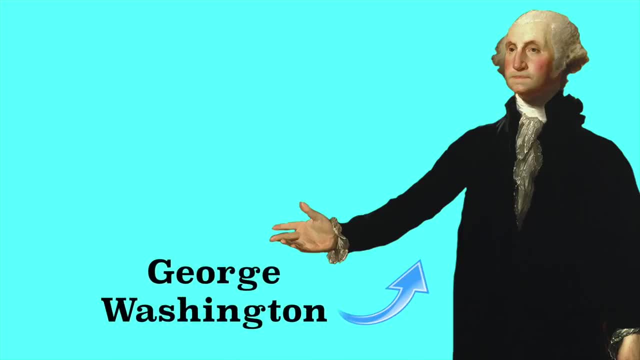 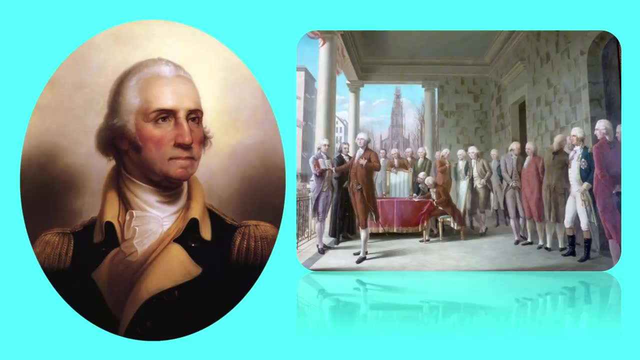 were Virginians Like this dude, George freaking Washington, who led the Continental Army. He led the Americans to victory at the Battle of Yorktown and later became the first president of the newly formed country of the United States. Jefferson and Madison were later. 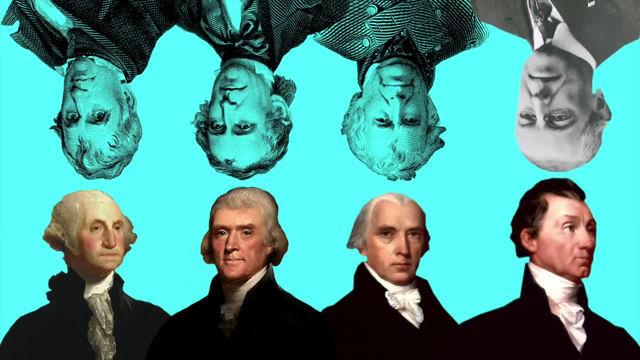 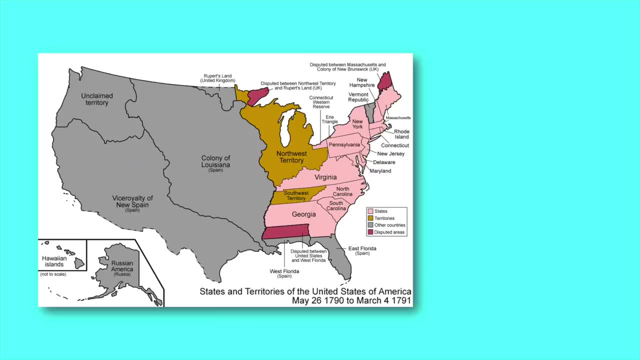 president-elected by the United States, Or this dude, James Madison, who, I don't know, was the next president as well. In fact, eight American presidents were born in Virginia In the early years of the United States being a country, the now state of Virginia. 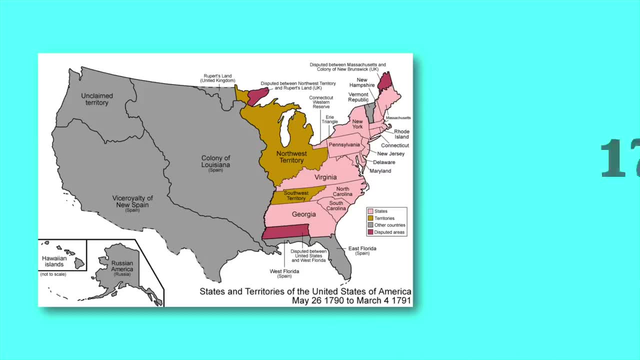 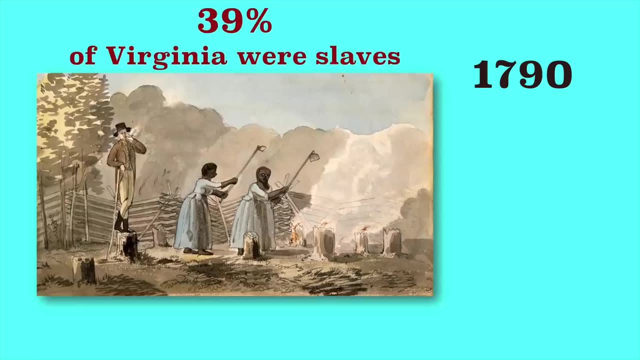 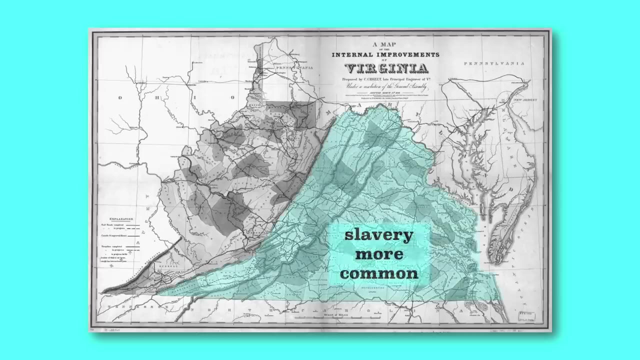 had the largest population by far. In 1790,, 19% of the whole country lived in the state. Also in 1790, more than 39% of the population consisted of slaves, But while slavery remained prevalent in eastern Virginia, 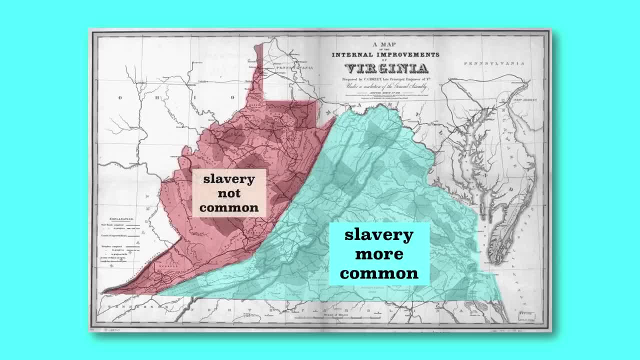 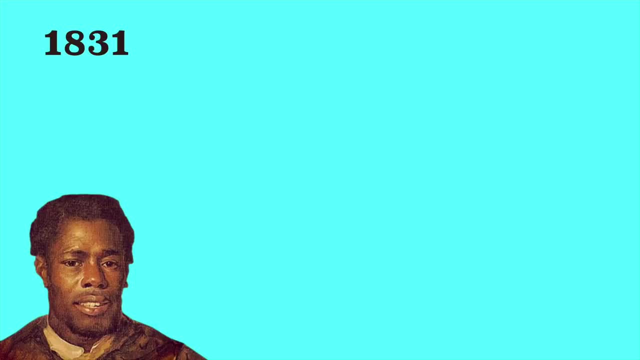 up until the end of the 19th century, the general Soviet state's own national democracy was typical for the state to JESUS. up in the mountains in western Virginia there were a lot less slaves and a lot more antislavery folks. In 1831, an enslaved preacher named Nat Turner led a slave rebellion. 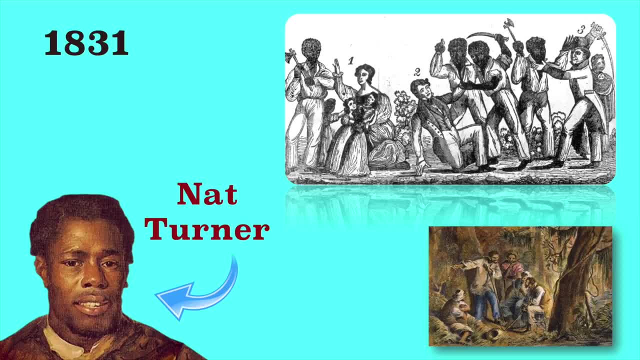 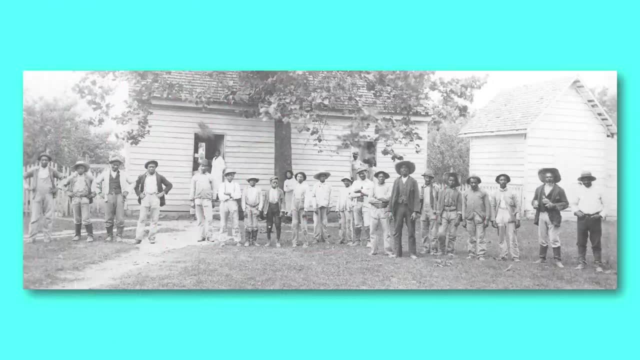 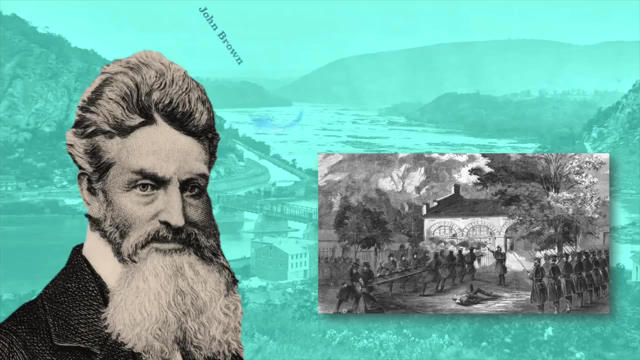 killing as many as 60 people. In response, around 30 African Americans were hanged or expelled from the state, and the General Assembly passed harsher slave laws, like laws making it illegal to teach slaves how to read or write. Virginia was also where the abolitionist John Brown tried and failed. 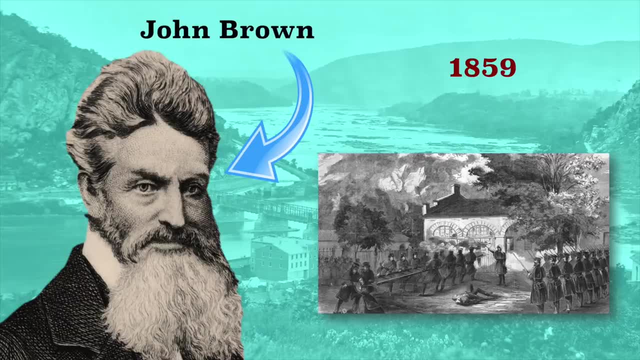 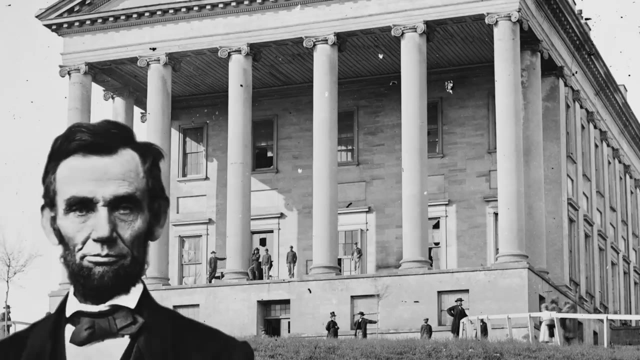 to incite another slave rebellion in 1859. He attempted to take over a federal armory at Harper's Ferry, but ultimately Brown was captured and executed. Virginia's government absolutely refused to get rid of slavery After the election of Abraham Lincoln as President. 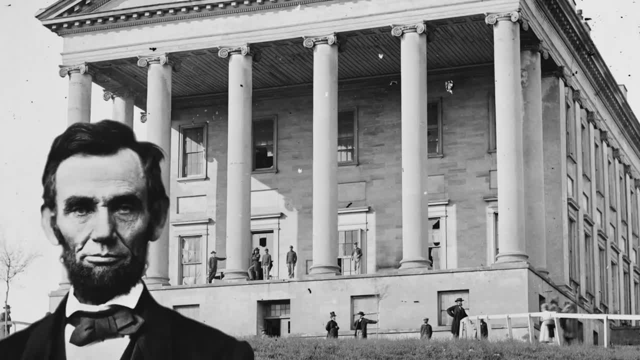 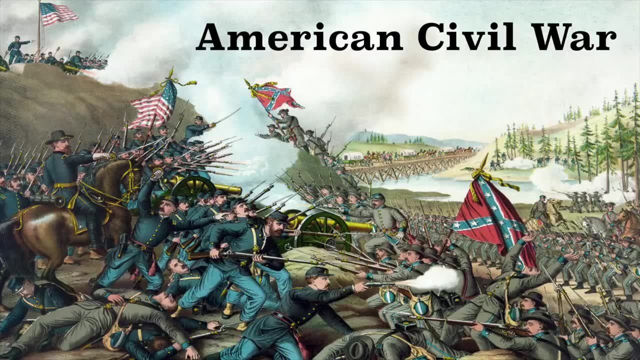 the General Assembly voted to secede from the Union over the issue, and this soon led to the American Revolution. The American Revolution was the first in the history of the United States to end the Civil War, with Virginia leading the fight for the newly formed Confederate States of. 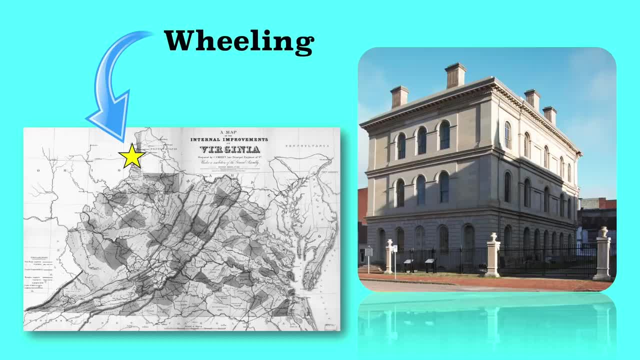 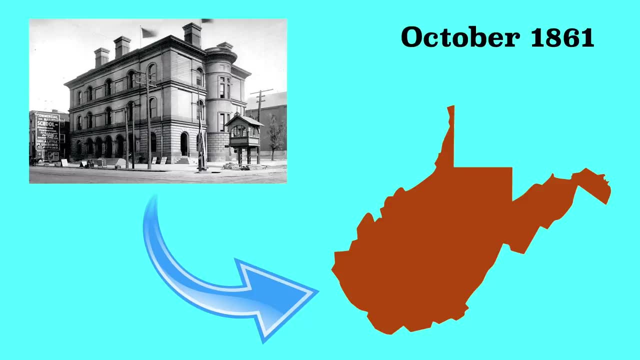 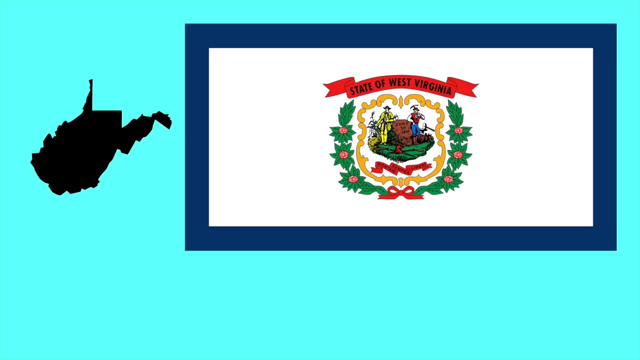 America. Several western Virginians in Wheeling, however, opposed secession and wanted to stay with the Union. In October 1861, they voted for a new state and the next April they had a new constitution. They were admitted to the Union as West Virginia on June 20, 1863. So this split. 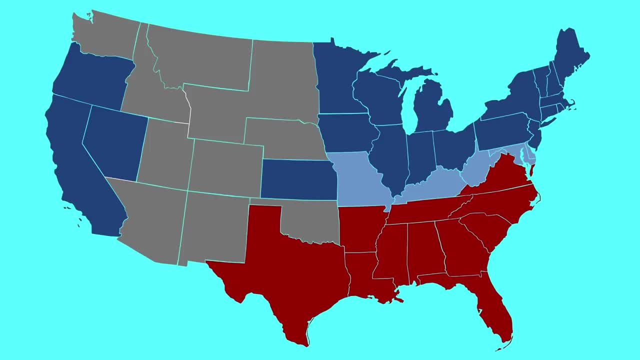 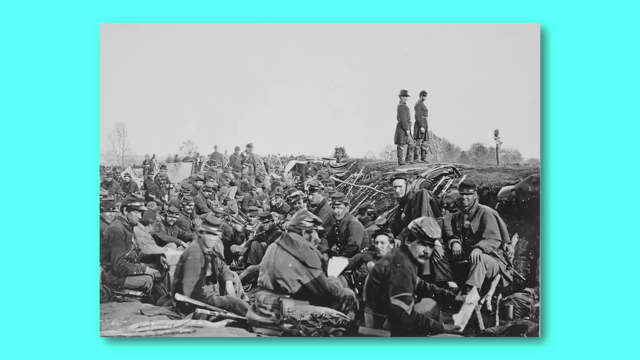 Virginia into two states, with West Virginia fighting for the Union and Virginia fighting for the Confederates, And it was basically a smaller version of the entire war. and boy were both states on the front lines of it. Many prominent Confederate generals like Jeb Stuart. 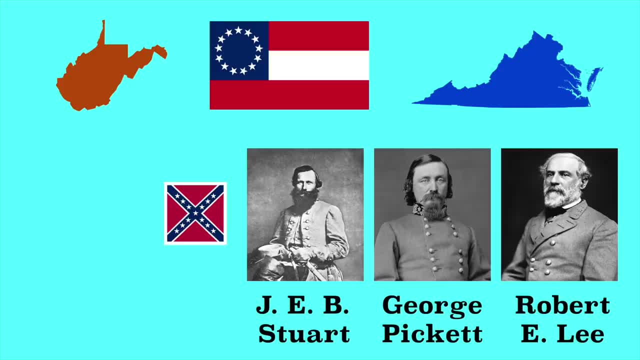 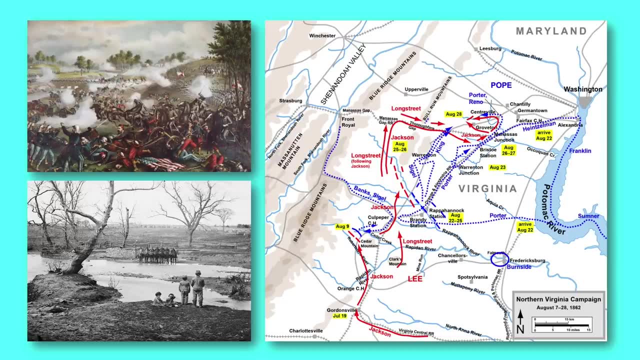 George Pickett and THE Robert E Lee were from Virginia and Stonewall Jackson was from what became West Virginia. Most of the battles in the eastern theater of the Civil War took place in Virginia. Most of the battles in the eastern theater of the Civil War took place in Virginia. 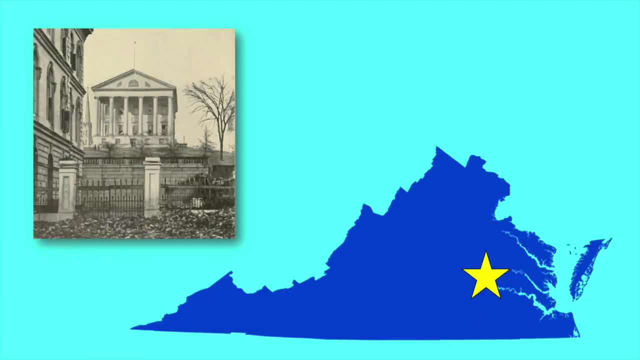 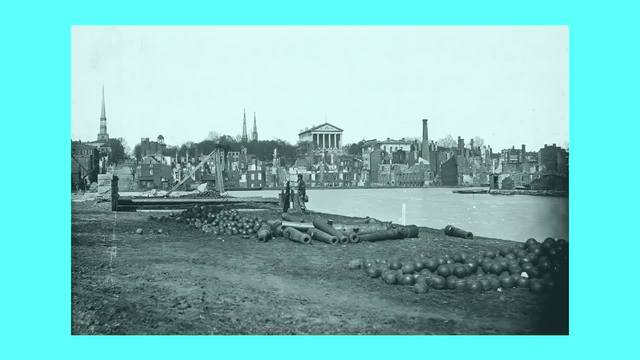 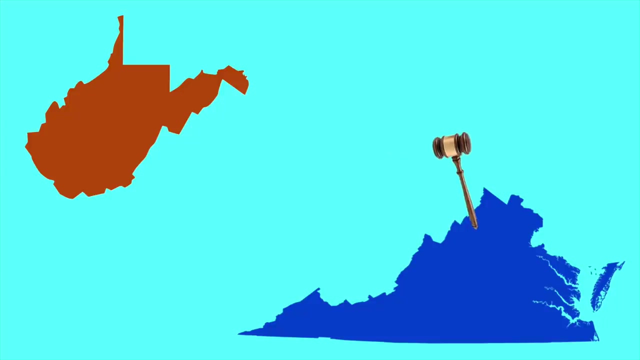 mainly since the Confederates had to defend its national capital there, which was Richmond, And there is no doubt that the Civil War left Virginia devastated. After the Confederacy lost the war and the United States reunited, Virginia sued West Virginia to get some of its counties back, but the Supreme Court said no. Virginia also tried to get West. 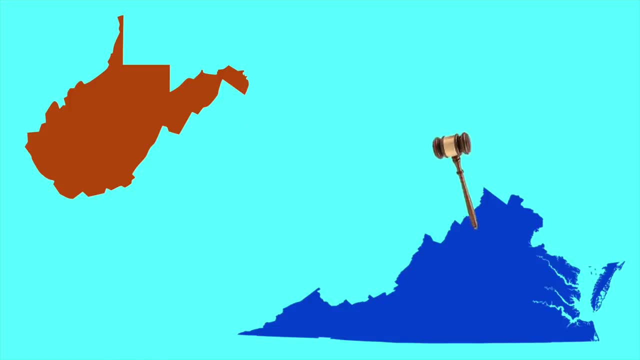 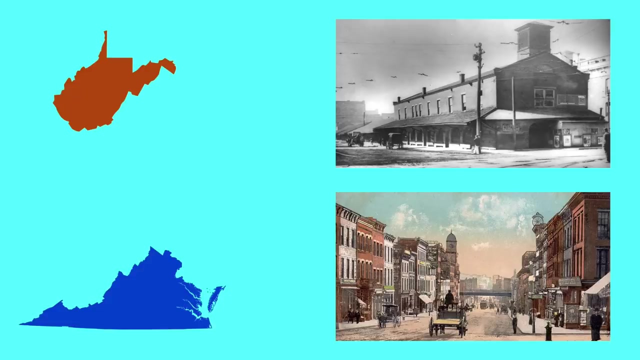 Virginia to pay off some of its Civil War debts, and this dispute lasted until 1911. When, finally, the Supreme Court did make West Virginia pay over $12 million dollars of Virginia Civil War debt, The economies of both states struggled for the rest of the 1800s, However. 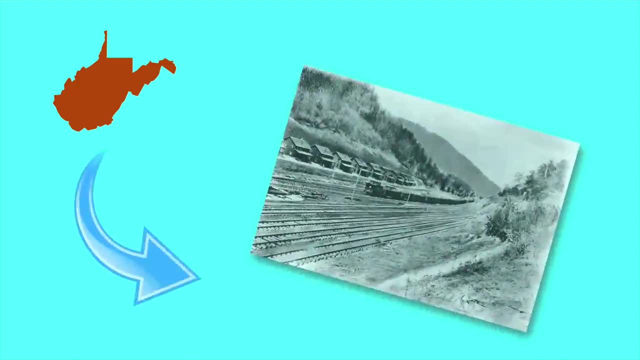 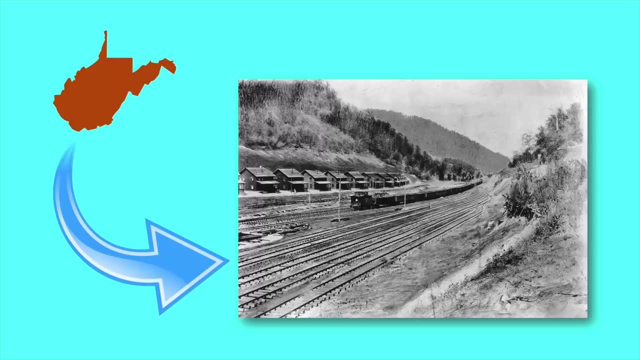 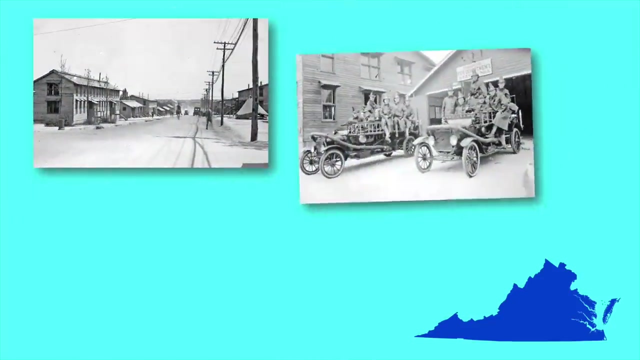 West Virginia's economy did start growing more quickly thanks to its plentiful natural resources, and both logging and coal mining expanded in the state. It wasn't until World War I when the economy really picked up in Virginia. that's when it got a boost from the 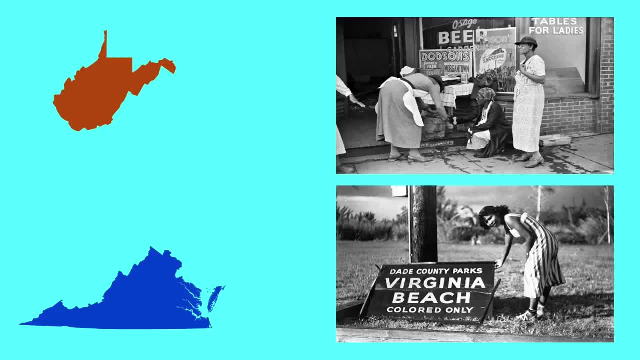 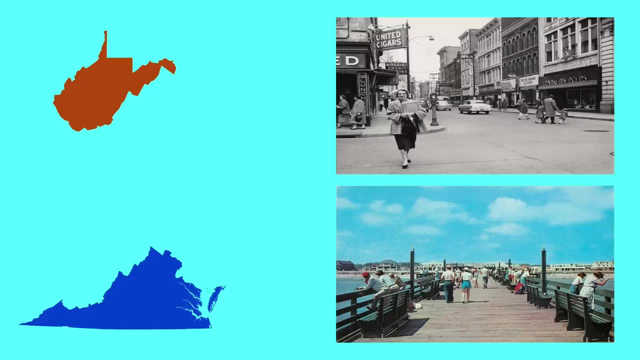 newfound federal spending for the military. Meanwhile, both states had racial segregation up until the 1960s. For the rest of the 1900s, Virginia's economy diversified a lot, while West Virginia's didn't nearly as much. Plus, 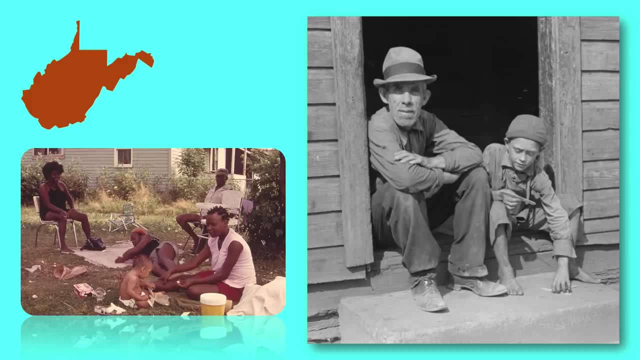 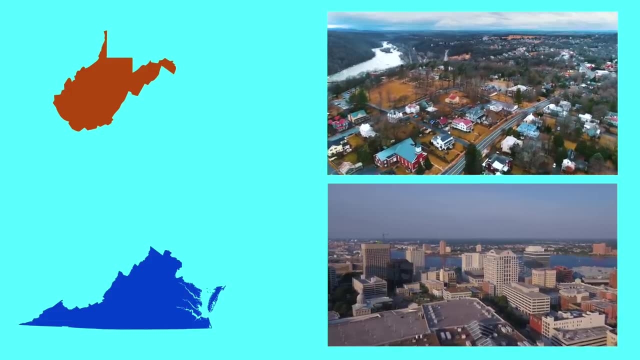 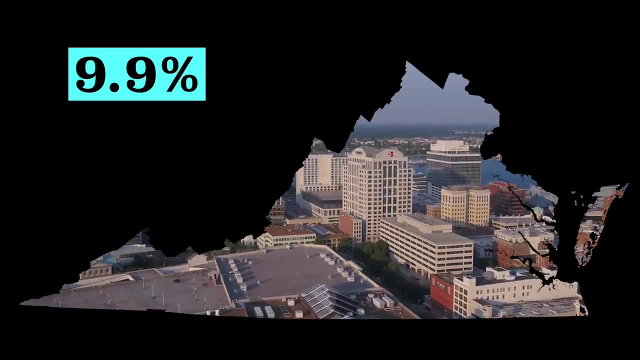 most West Virginians eventually sold their rights to land and minerals to large corporations. Today, this is the main reason why both states are actually quite different. West Virginia has one of the highest poverty rates in the country, while Virginia has one of the lowest. 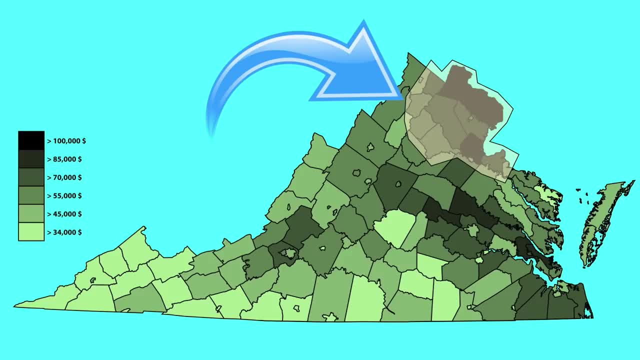 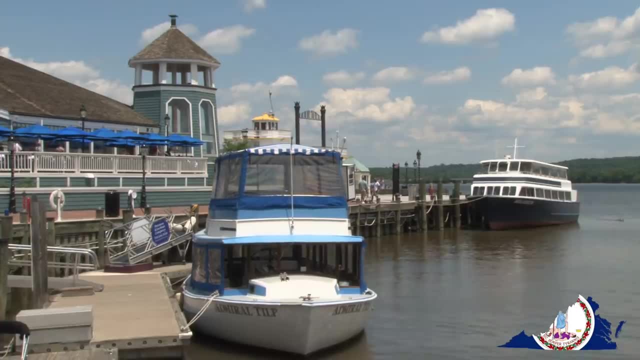 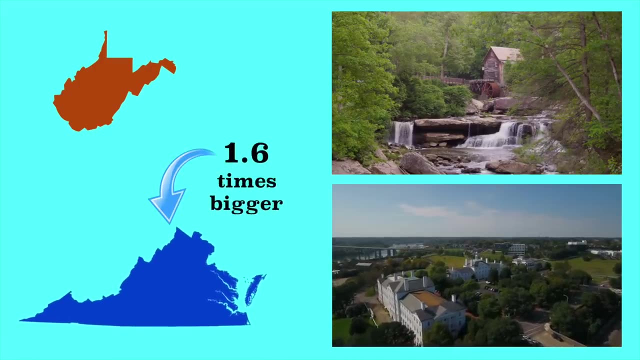 poverty rates in the country. Now, this is mostly due to the concentration of wealth in northeastern Virginia, in the suburbs of Washington DC- All those lobbyists up there- am I right? Okay, what about other differences? Well, first of all, Virginia is about 1.6 times. 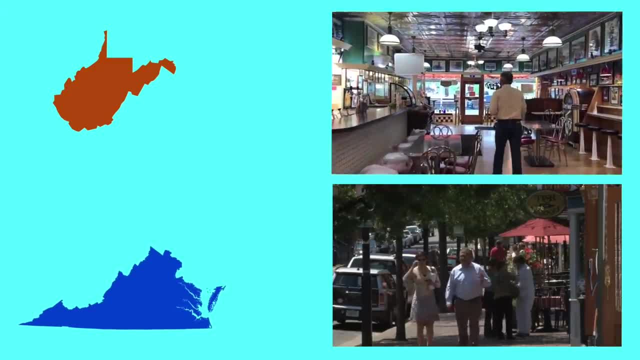 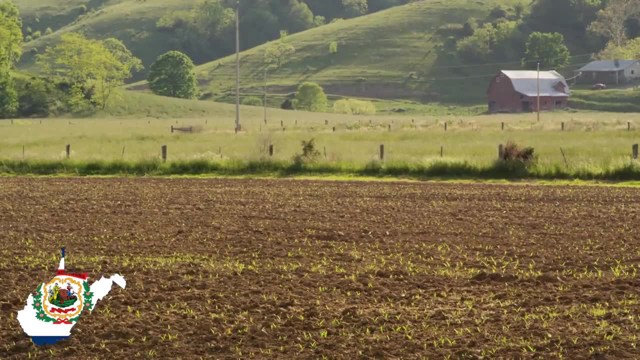 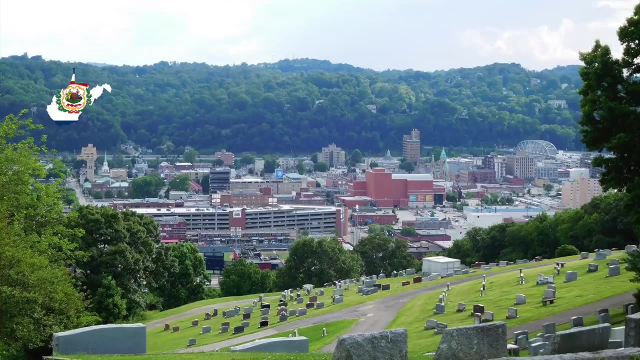 bigger in land area. Virginia also has a lot more people. In fact, it has nearly five times as many people. While West Virginia's population has actually been declining in recent years, Virginia's population continues to steadily increase. In fact, West Virginia lost a higher percentage of its residents than any other state in the country. 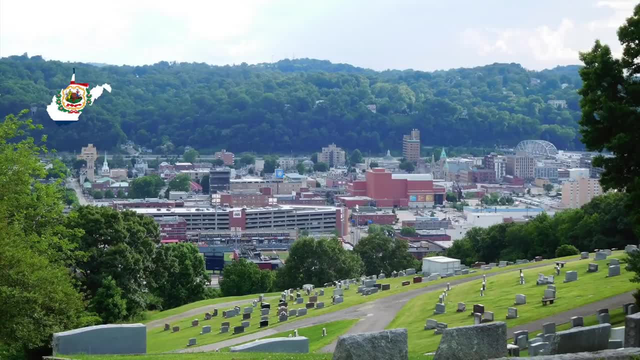 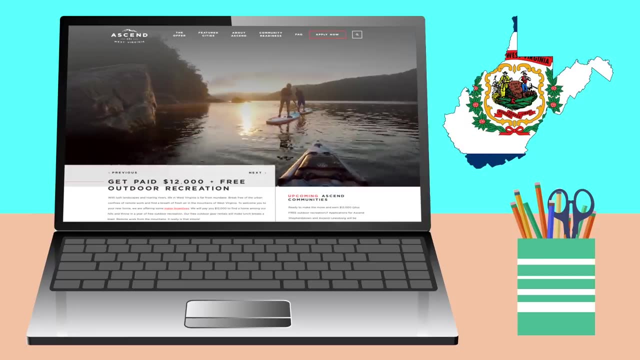 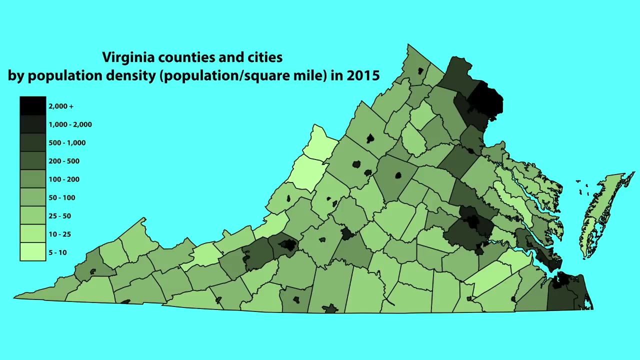 over the past ten years and currently has fewer residents now than it did in 1950.. To solve this potential crisis, West Virginia will currently pay you $12,000 to move there. Virginia has a higher population density. West Virginia has smaller cities. In fact, its largest city, Charleston. 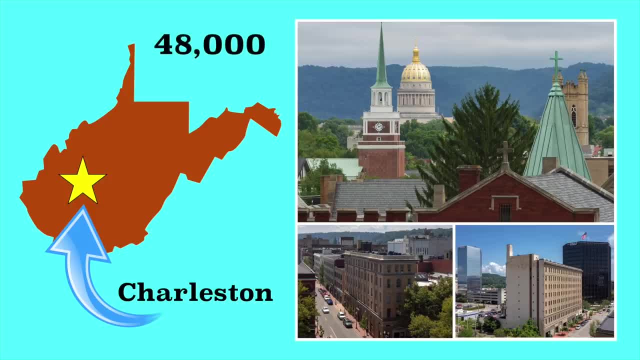 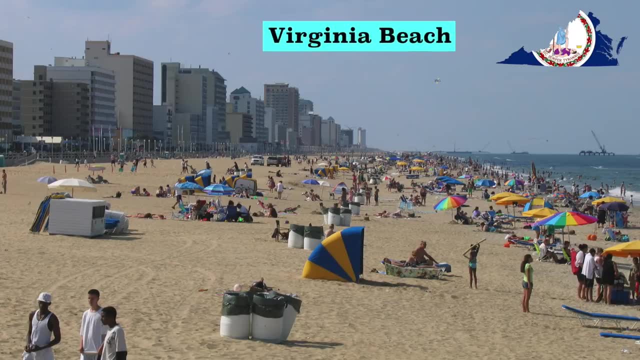 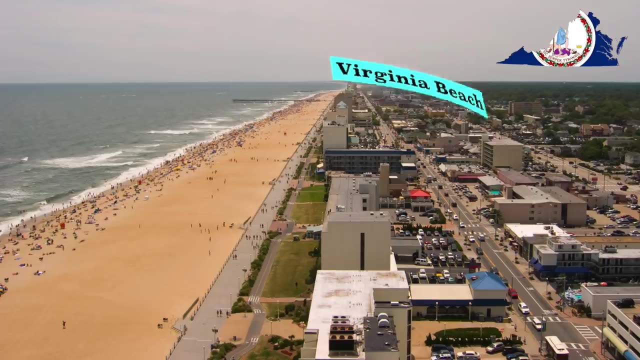 which also happens to be its capital, has only 48,000 people. Yeah, it used to have more than 85,000 in 1960.. Virginia's biggest city is Virginia Beach, which has around 450,000 people. By the way, Virginia Beach does have the world's longest tourist beach. I've been there and it does seem to go on forever. That said again, Virginia also has part of the Washington DC metropolitan area and that has 5.4 million people. It's one of the wealthiest and most educated metro areas. 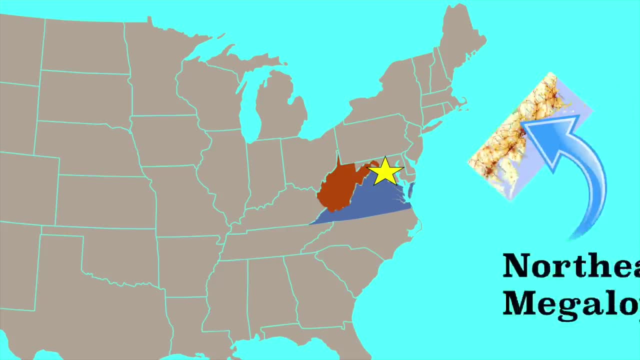 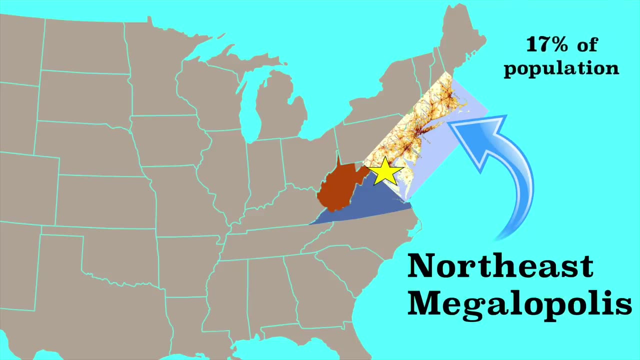 in the country and marks the southern end of the northeast megalopolis, a part of the country that contains more than 17% of its entire population. Virginia is the largest city in the United States, with a population of more than 50 million people on less than 2% of the country's land area. 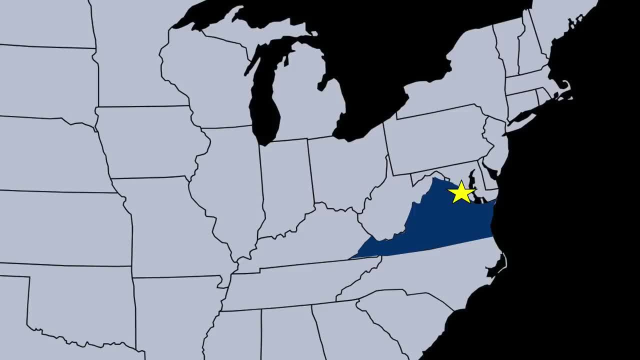 Virginia borders more states. In addition to bordering the District of Columbia, which is not a state, of course, and West Virginia, Virginia also borders Maryland, Kentucky, Tennessee and North Carolina. West Virginia also borders Maryland and Kentucky, but also Pennsylvania and Ohio. Virginia residents are younger. Virginia has a much. 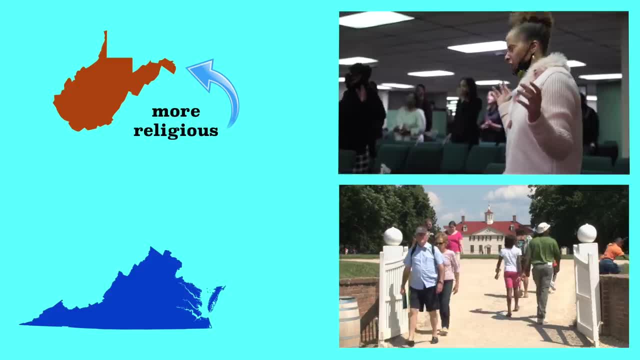 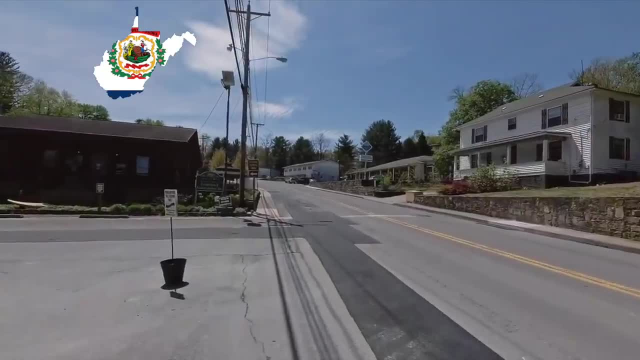 more ethnically diverse population. Virginia has a much more diverse population. Virginia residents are younger. Virginia has a much more ethnically diverse population. West Virginia residents are more religious. The violent crime rate is lower in Virginia. However, West Virginia's violent crime rate has been falling in recent years. More Virginians have college degrees, but West Virginia spends more per student on education, so take that Virginia. Oh yeah, According to Forbes Magazine, Virginia is a much better state to do business in and is ranked 4th in the country, compared to West Virginia being ranked 2nd. 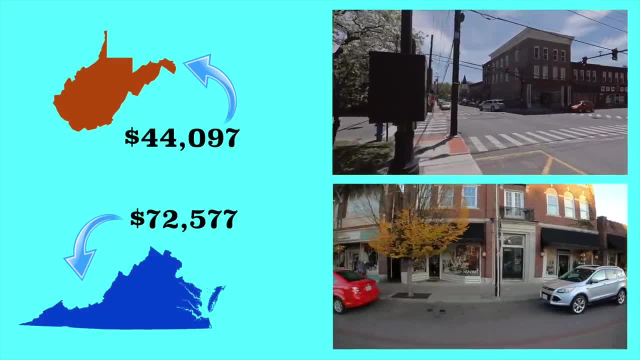 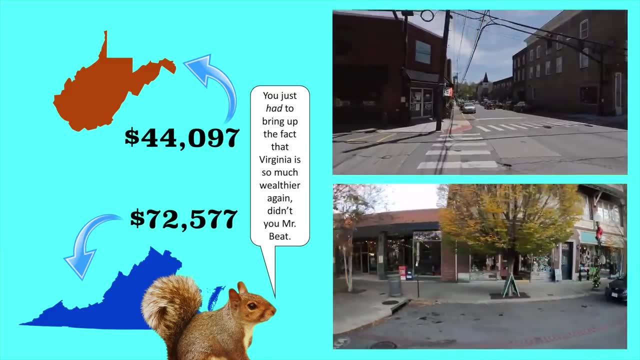 Related to this, the median household income is much higher in Virginia. You just had to bring up the fact that Virginia is so much wealthier again, didn't you, Mr Beat? Well, I'm sorry. Oh, just stop dunking on states, okay. Uh, okay, Let's see How shall I carefully proceed. Oh, I know West Virginia has a much lower cost of living, eh? Major industries in Virginia, including solar agricultureowym션s, hardware and the like, include health care. 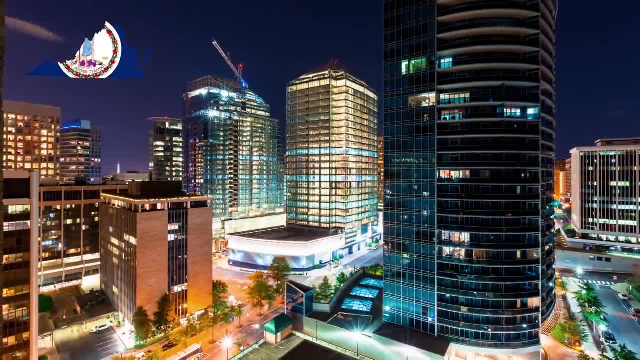 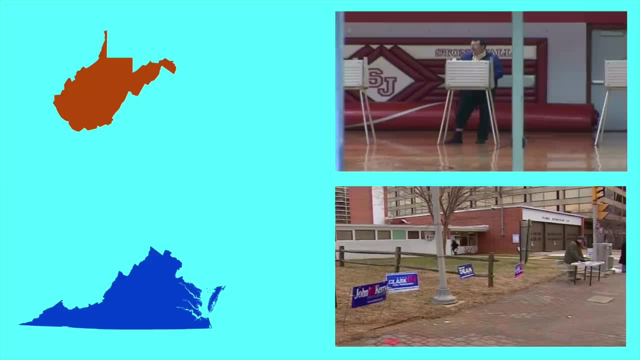 government and public services and technology. We'll talk about both in a minute. Lots of federal agencies have headquarters in the state. Major industries in West Virginia include manufacturing, energy and tourism. Parking or other. publicvery is a мой job. West Virginia residents tend to be more conservative. Indeed, Virginians tend to vote more for Democratic Party candidates in recent years. Both of Virginia's senators are Democrat, has one Republican and one Democrat Senator, but that Democrat is Joe Manchin, who has gotten a lot of attention this year for often being a swing vote that sometimes 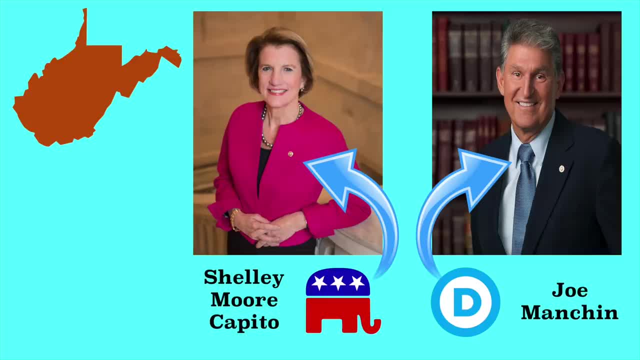 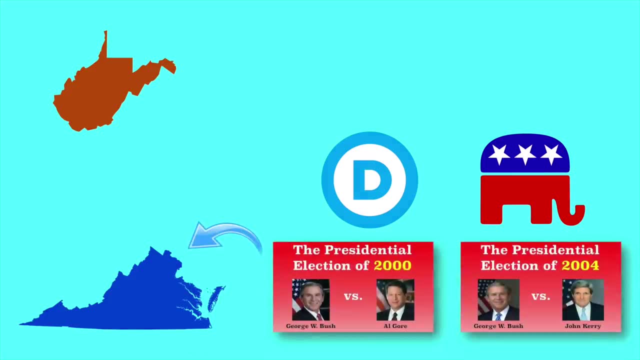 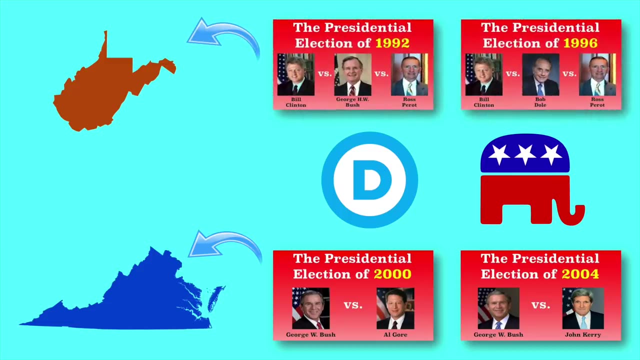 votes against his fellow Democrats on bills. Historically, however, both states have gone back and forth between the two major political parties. After all, Virginia voted for George W Bush for President in 2000 and 2004, and West Virginia voted reliably for Democrats. 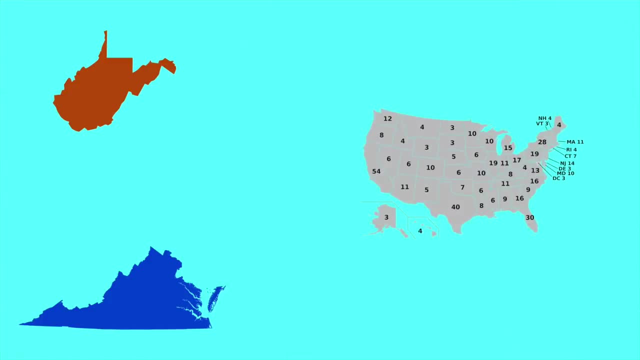 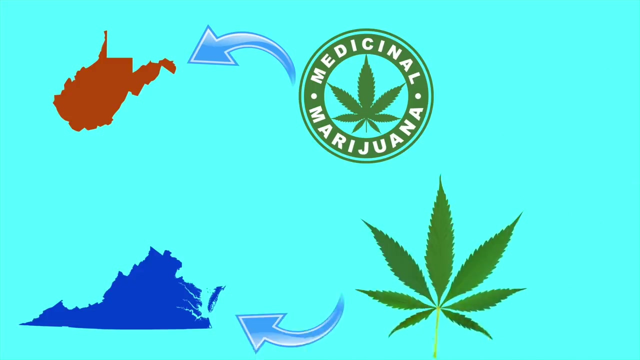 before the 2000s. Speaking of presidential elections, Virginia has 13 electoral votes and after the 2020 Census, West Virginia is going from 5 to 4.. Taxes are lower in Virginia. While medical marijuana is legal in West Virginia, recreational marijuana is legal. 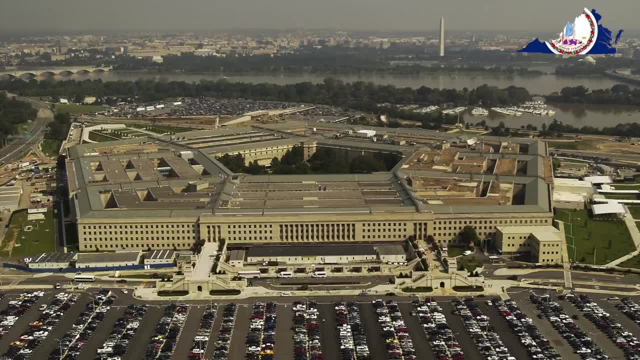 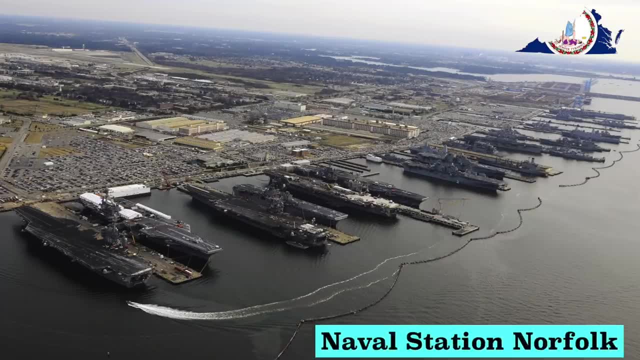 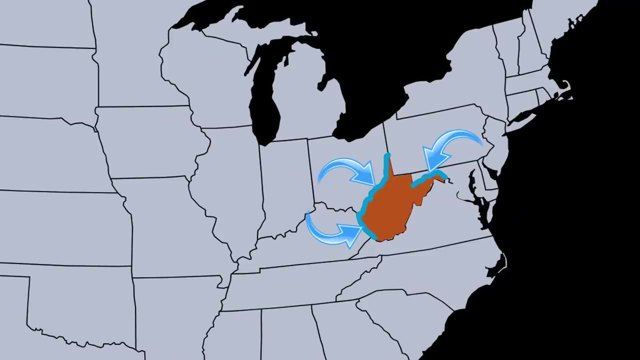 for all adults in Virginia. Virginia has the largest office building in the world, the Pentagon, Oh, and the largest naval base in the world, Naval Station Norfolk. in uh, Norfolk, Three different rivers make up part of the border of West Virginia, But also humans created its borders, so that's why it looks so weird and 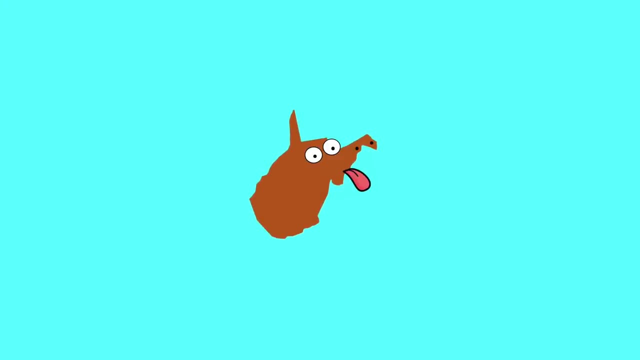 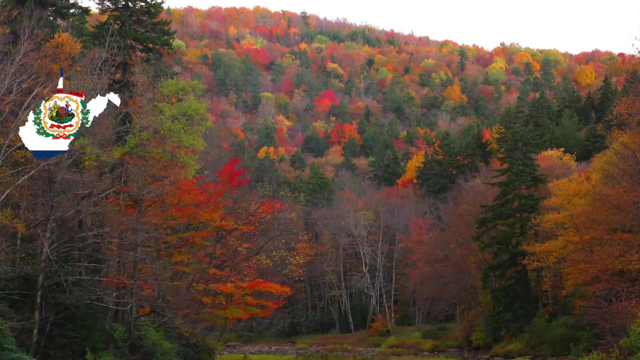 is so difficult to draw freehand. Go ahead and do it and try. I dare you. West Virginia is simply more beautiful. I mean freaking. look at that. It has more wilderness and is the third most forested state in the country, after Maine and New Hampshire. 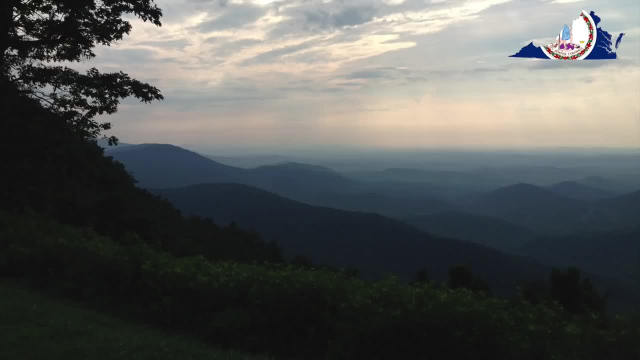 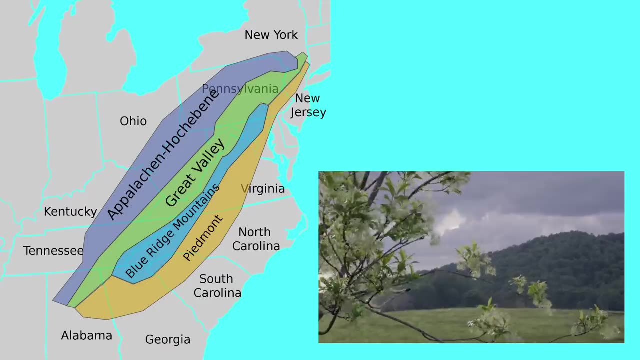 Virginia is the number one mostійсьed state in the world. Virginia też przep Tischler��. While both are considered Mid-Atlantic states, only Virginia borders the Atlantic Ocean. Also, while both are, at least in part, of the. 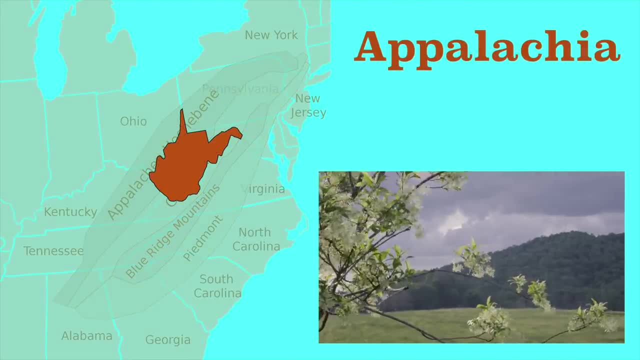 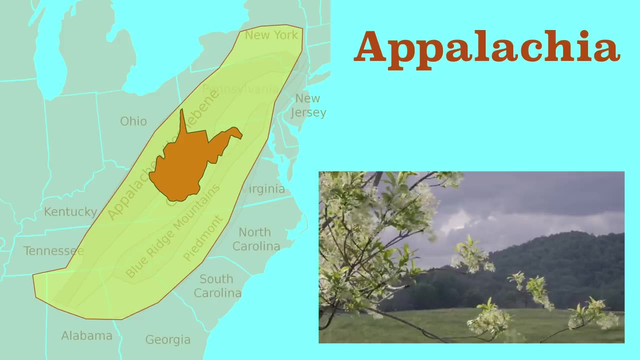 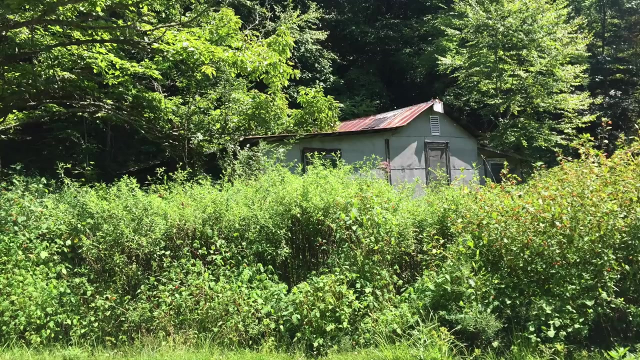 Appalachian region. West Virginia is the only state entirely in Appalachia, a cultural region that surrounds the Appalachian Mountains all the way from Mississippi to New York. While this region has historically held lots of natural resources, it also has, unfortunately, been associated with lots of poverty. As I mentioned earlier, West Virginia has struggled. 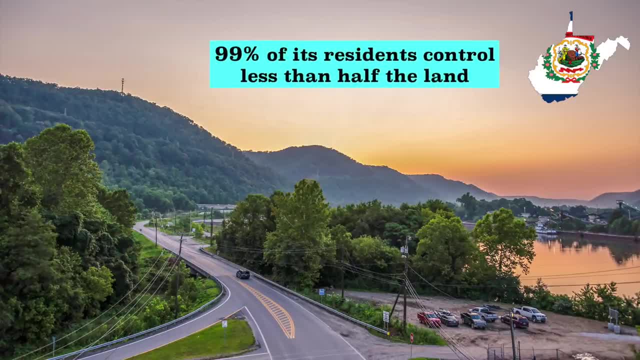 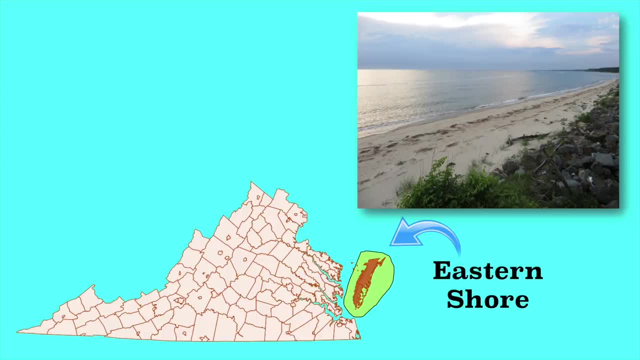 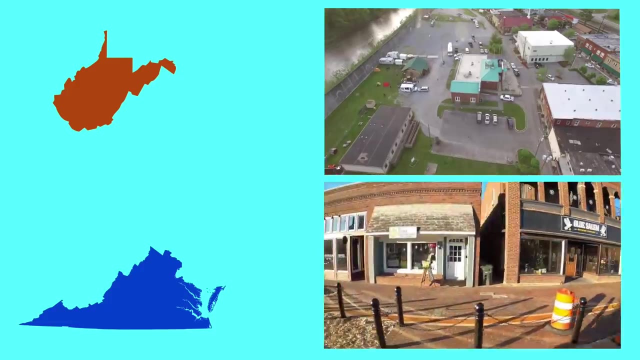 and today, 99% of its residents control less than half the land. Oh yeah, and people often forget about Virginia's eastern shore, the only part of the state not connected by land. You can still drive across the Chesapeake Bay, however, via the Chesapeake Bay Bridge Tunnel. Hey, let's end this. 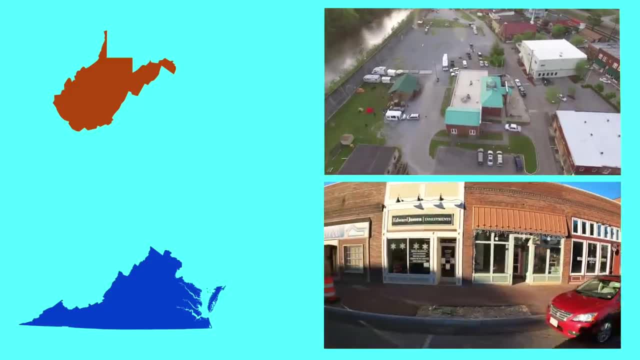 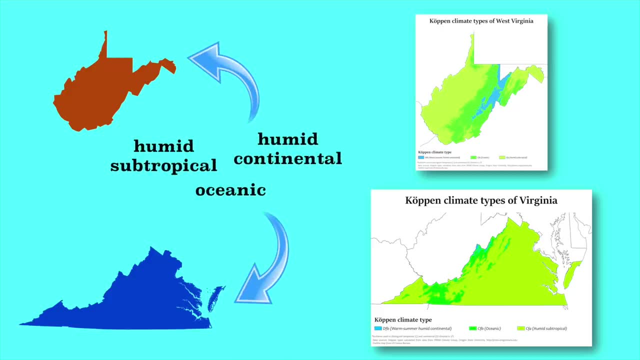 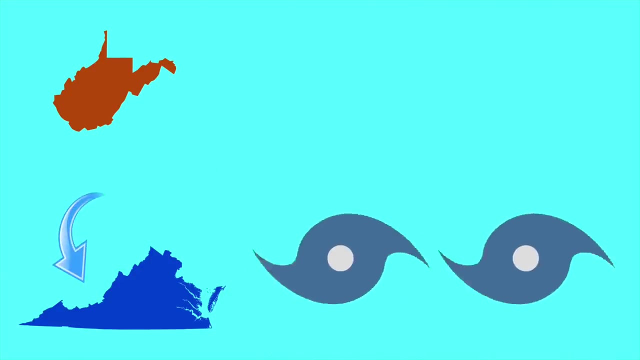 video with similarities? I guess there aren't many. Both are mid-Atlantic states. Oh, I already said that Both states have oceanic, humid, subtropical and humid continental climates. Being near the ocean, Virginia does have to worry about hurricanes and West Virginia does not. 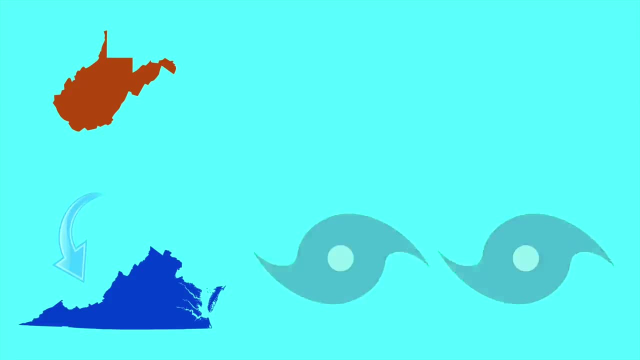 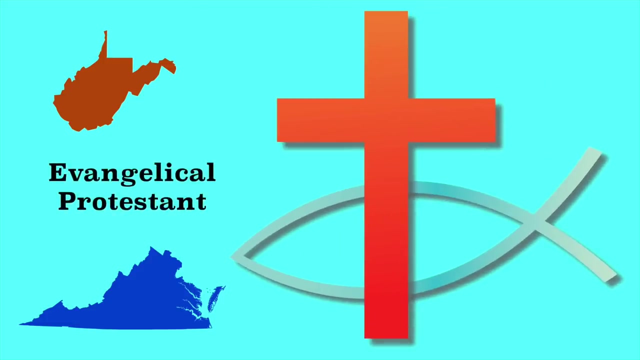 Wait a second, I thought we were doing similarities here. Okay, there are no professional sports teams in either state, but many of their college teams are big in the NCAA Division. I baby. The biggest religion in both is Christianity, specifically Evangelical Protestant. Both have exactly one national park- Residents of both. 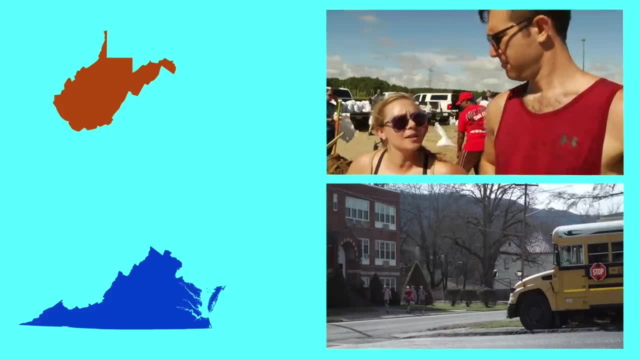 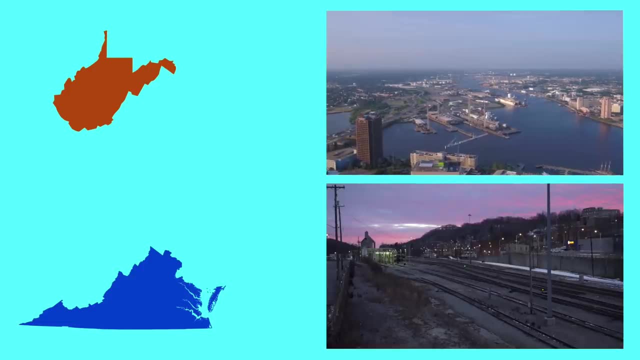 definitely have a Southern-type accent. I mean, that's kind of it. That's all I can think of at the moment. anyway, What am I missing? Overall, both states are definitely wonderful places. Virginia obviously has all the history and beauty, West Virginia- 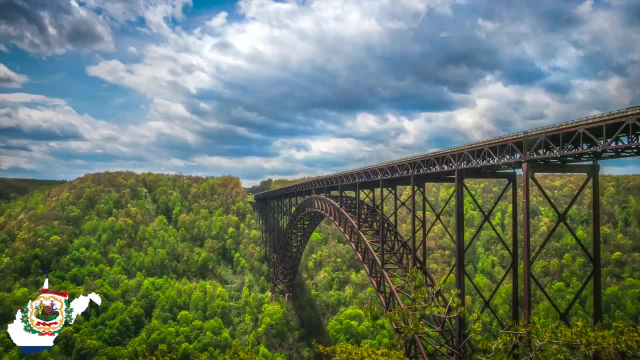 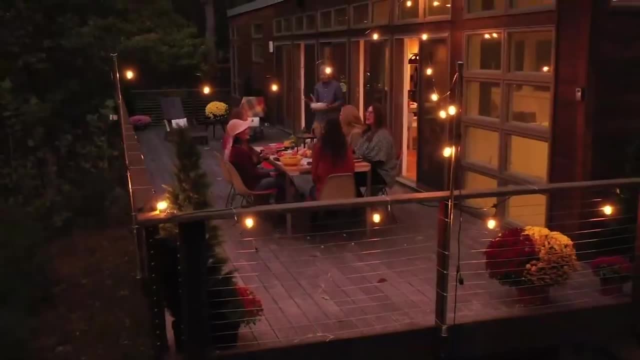 clearly has the beauty and might not look as good as Virginia based on this video, but, like I said earlier, they'll now pay you to move there. If you work remotely, you might move there now, before things heat up and the cost of living skyrockets like it has been. 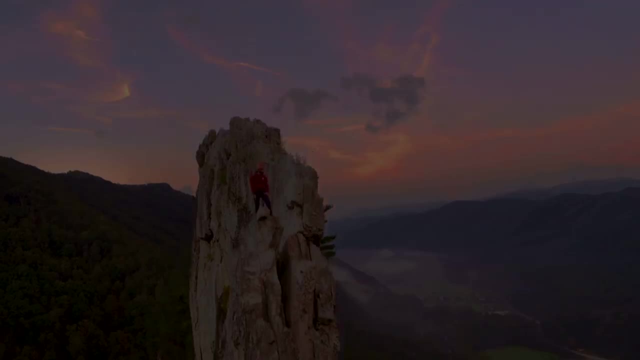 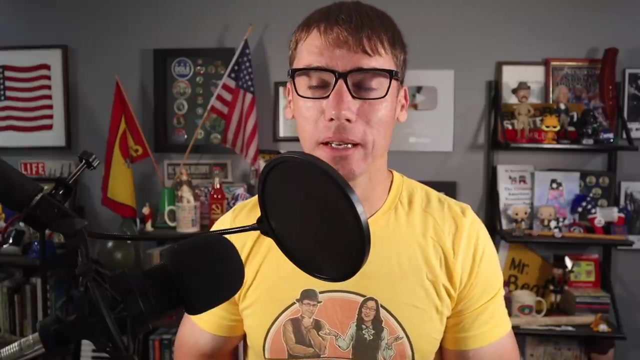 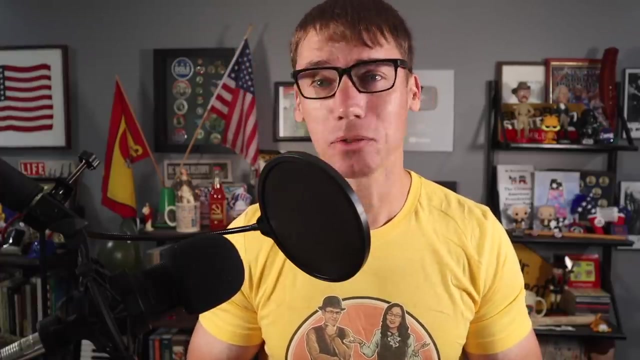 in most other places I know. I know I made a lot of folks upset by deciding to compare Virginia and West Virginia instead of Virginia and Maryland, but I had a lot of folks that wanted to see West Virginia and Virginia dang it And I could always later on still compare Virginia and Maryland. 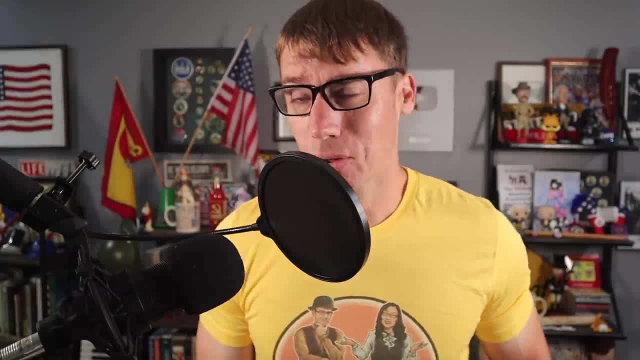 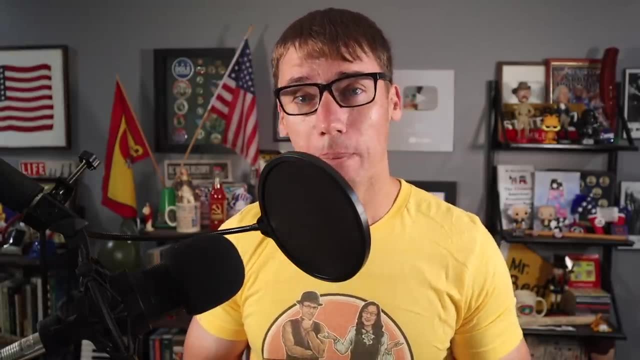 It's my channel, I can do what I want. So what other states should I compare for this series? I know I'm running out, but there are still a few left. Let me know down below. and now it's time for my monthly shoutout to all my Patreon supporters who donate at: 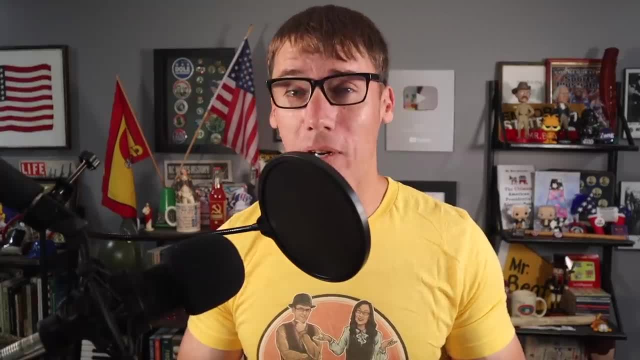 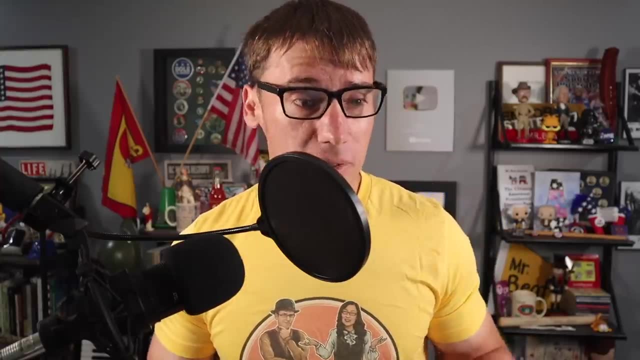 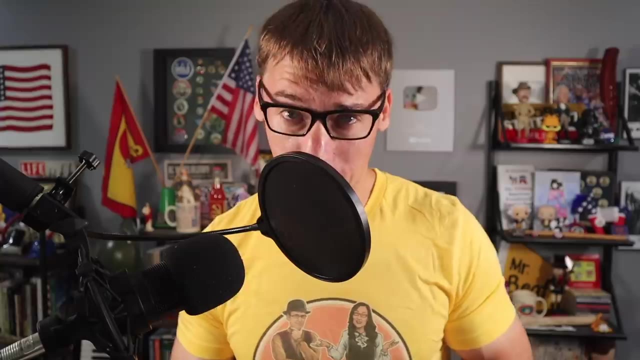 least ten bucks or more each month to my channel, starting with my biggest donors at the channel at the George Washington level: Alicia Solberg, Andrew B, Austin, Siros, Brady Bardwell, Dr Paul J Lilly, Matt Standish, Nick Everett, Sean Conant and Will Scruggs At the Grover.